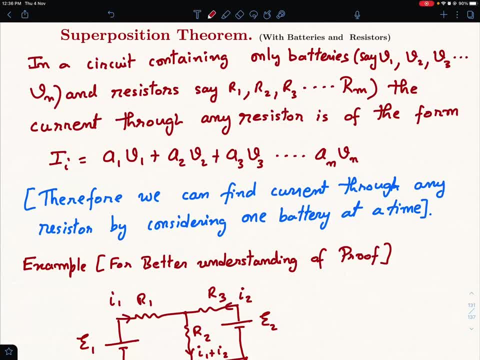 Hello viewers, welcome to my channel, IIT Jai, Olympiads and AP Physics with Ambarish. First of all, wish you all a very happy Diwali. One of my subscribers had requested me to make a video on superposition theorem and the proof of the superposition theorem, So here it is. 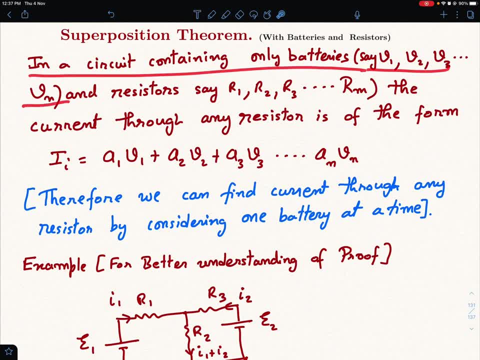 I am presenting the superposition theorem today. So what is the statement of the superposition theorem In a circuit containing only batteries say V1, V2, up to Vn, and resistors say R1, R2, R3 and up to Rm. the current through any resistor is of the form A1, V1 plus A2, V2 plus A3, V3. 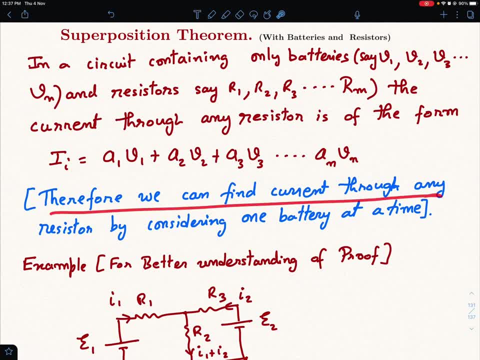 all the way up to An Vn Here. V1,, V2, V3, etc. are the emfs of all the batteries. Therefore we can find current through any resistor by considering one battery at a time. So it is a linear function of various 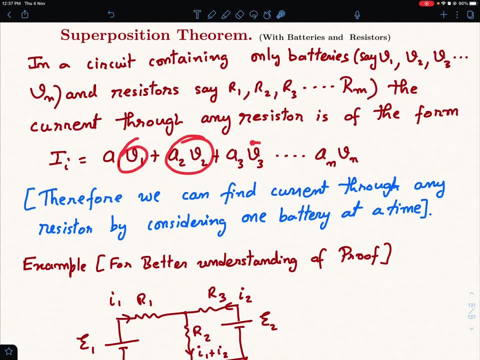 emfs. So, for example, to calculate the first term, I can just put all these terms to 0, right. Similarly, to calculate the second term, I can put V1, V3, etc. all the way up to Vn equal to. 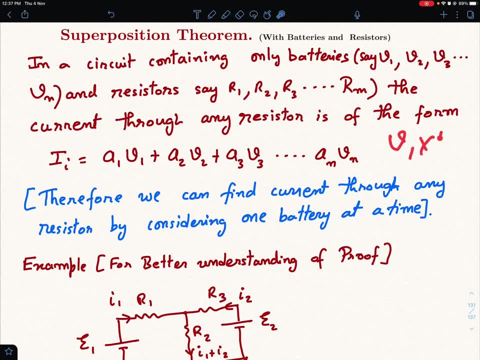 0. Similarly, I can consider the role of one battery at a time to get this. Why we can do that? That is because there is no term of the form V1 into V2.. That is the beauty of linearity. because of the our system, If the solution is a linear combination of all the emfs, 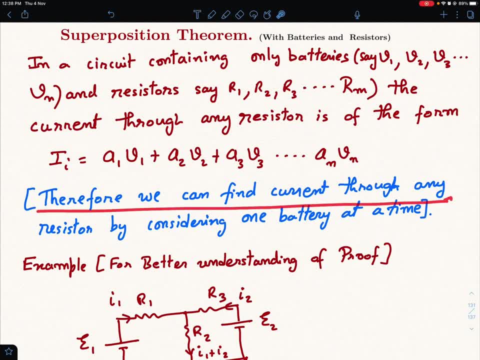 and there is no term containing V1 into V2, so therefore we can consider the role of one battery at a time. That is what I have written. Therefore, we can find the current through any resistor by considering one battery at a time and considering all other batteries. 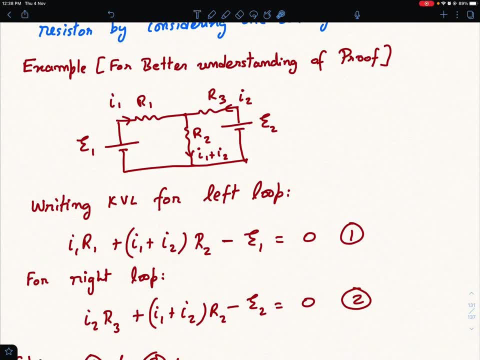 as short circuits, right? So for the proof, before I get into the proof, I will just motivate the proof by an example so that you can easily understand my logic of the general proof. So let me just take a simple example. ok, So let us say I have a simple circuit like this: there is a battery. 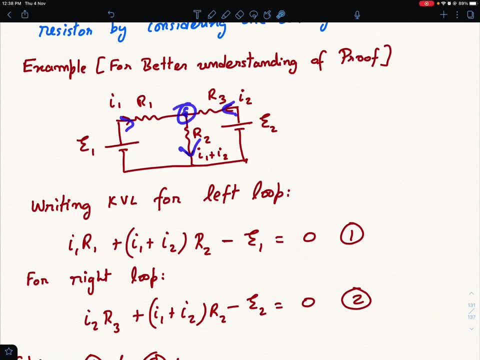 E 1, another battery, E 2. then there are 3 resistors, R 1, R 2 and R 3, and there is current I 1 here and there is current I 2 here, and I have satisfied the junction law here and there is the current. 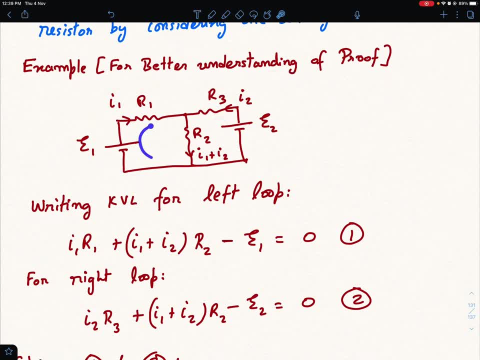 I 1 plus I 2.. So I have two unknowns and I have two loops. So there is this loop and there is this loop. So two unknowns and two loops, I can make the equation. So first equation: 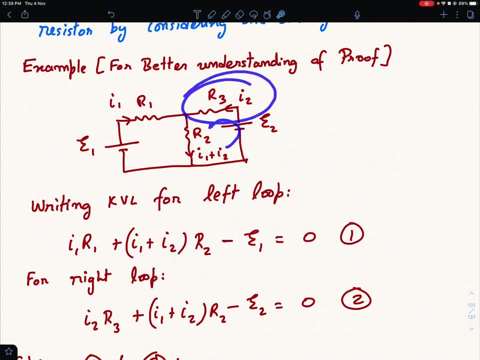 this loop: I 1, R 1 and plus I 1 plus I 2 into R 2 and then minus E 1, equal to 0.. Similarly for the second loop, I 2 into R 3, then I 1 plus I 2 into R 2 and minus E 2 is equal to. 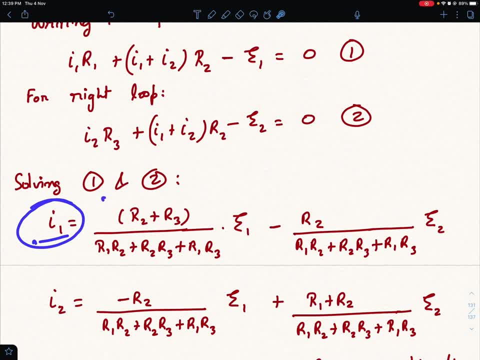 0, and now this is two variables and two equations we can easily solve, and if you solve you will get. this is the result for I 1.. So what you are seeing for I 1, there is some function of resistors, and then there is multiplication by E 1 and then again there is some function. 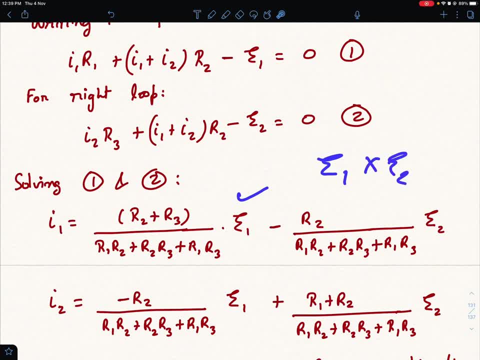 of resistors, and then there is multiplication by E 1, and then again there is some function of resistors, and then there is multiplication by E 2.. So what do you see? I 1 is a linear combination of E 1 and E 2.. There is no term like E 1 into E 2 or E 1 square or E 2 square. 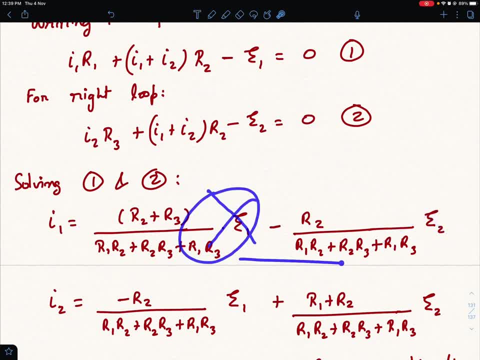 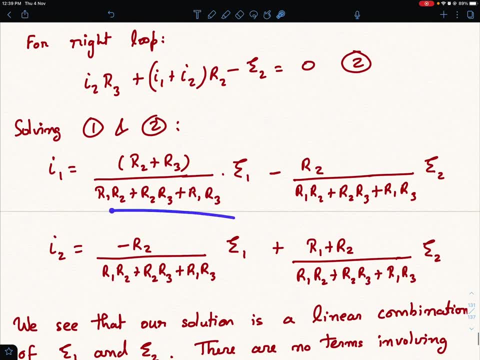 and therefore, for calculating the first term, I can put E 2 equal to 0 and calculate the first term, and then, for calculating the second term, I can put E 1 equal to 0 and calculate the second term, and then add the two terms to get the total current. 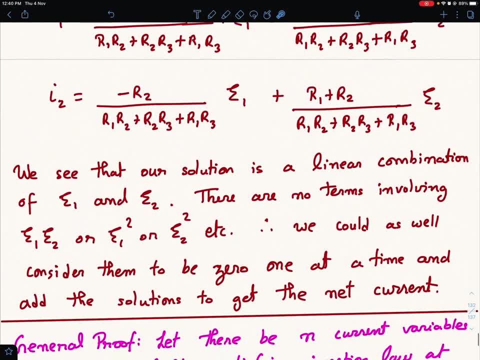 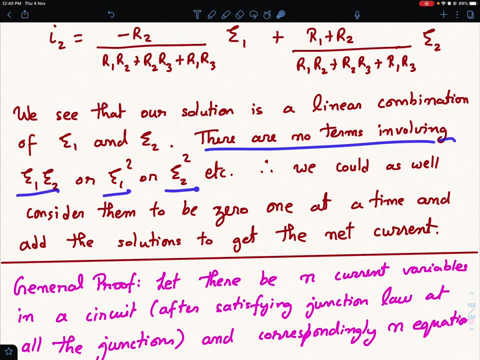 And similarly for I 2 also. you can see that it is going to be a linear combination of E 1 and E 2.. There is a pure resistor function and there is there is also pure resistance function. So we see that our solution is a linear combination of E 1 and E 2.. There 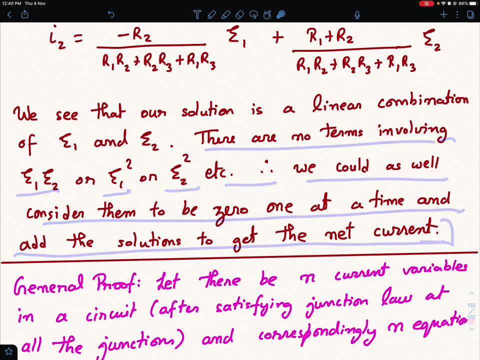 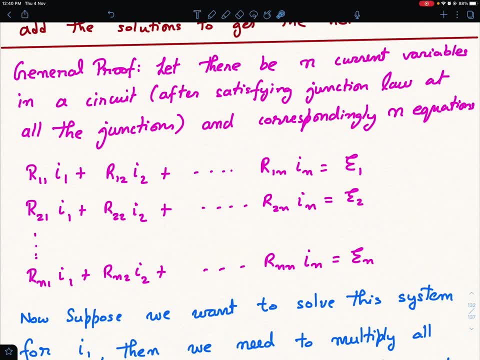 are no terms involving E 1, E 2 or E 1 square or E 2 square, etcetera. We could as well consider them to be 0, 1 at a time and add the solutions to get the net current. So if you have understood, 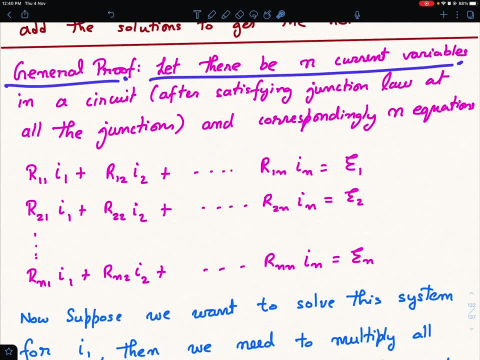 this example, then it should be simple extension towards the general proof. So let us get into the general proof now. Let there be n current variables in a circuit, after satisfying the junction law, at all the junctions. So if you satisfy the junction law, you will be able. 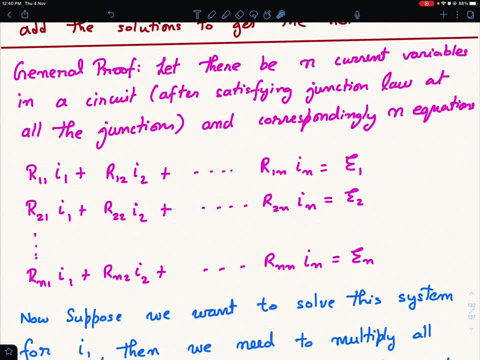 to see that as many loops are there as there will be as many current variables for a general circuit, and then we can make the corresponding n equations for each loop. So what will be the form of equations? See, in any loop there will be some current and 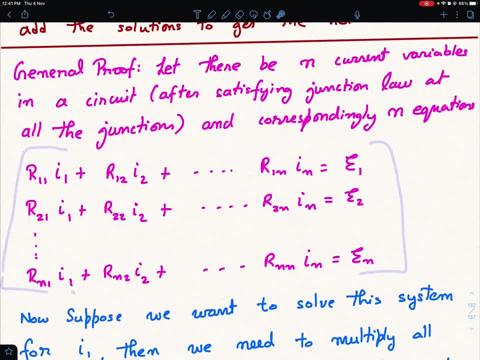 multiply by some resistance and some current multiply by some resistance and this will be equal to the emf in the general proof. Yeah, For the general proof. that is what we know now, because in the general proof if you have the logical expectation for a short circuit, 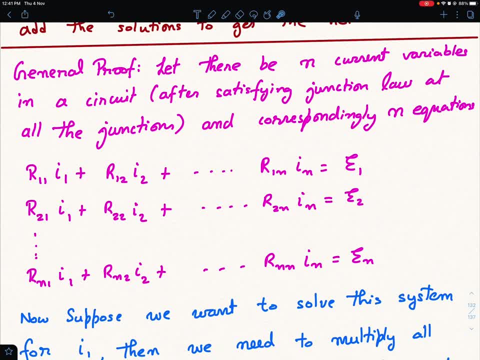 loop. So this is the form that equations are going to take. So there will be some coefficient of I 1, which is a function of resistors resistances. So let the equations be R 1 1, I 1 plus R 1 2, I 2. 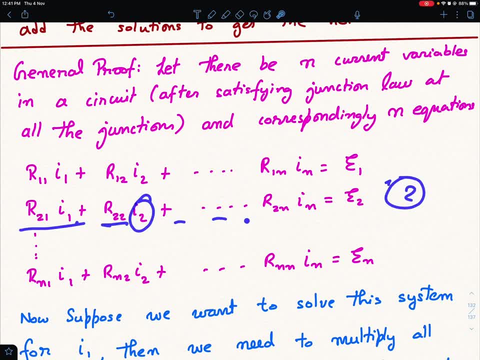 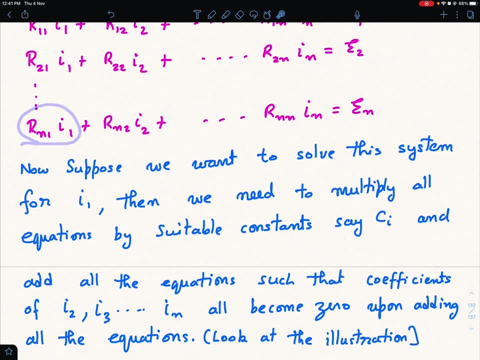 and so on, R 1 and I n is equal to E 1.. Similarly, the second equation for the second loop equation may be R 2: 1 into I 1, plus R 2, 2 into I 2, and so on, up to R 2 n into I n, equal to E 2.. Similarly, 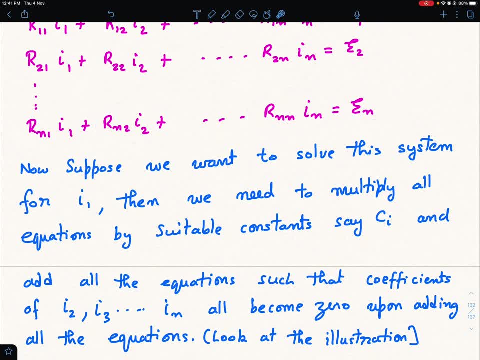 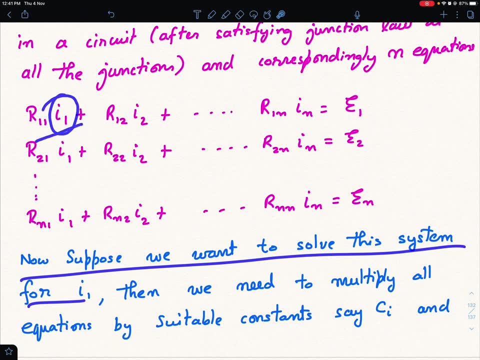 for nth loop. it could be R n 1 into I 1 plus R n 2 into I 2 and so on up to R n n into I. n is equal to E n. Now suppose we have to solve the system of equations for I 1.. Suppose I am focusing on 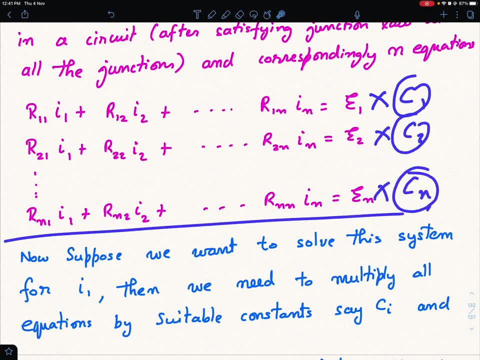 how to solve for the variable I 1.. Then what will I do? I will multiply all these equations by suitable constants and then add them up so that the coefficient of I 2 becomes 0 in the addition and all the all the other coefficients will be 0 in the addition. So I will multiply all these. 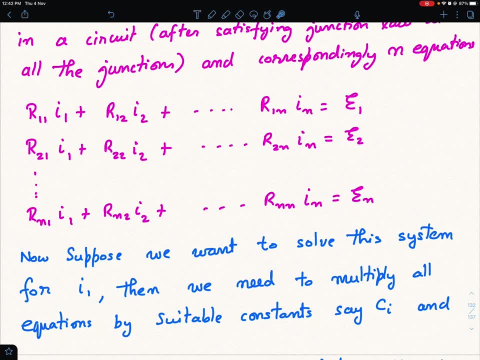 coefficients by suitable constants and then add them up so that the coefficient of I 2 becomes 0 in the addition. So I will multiply all these coefficients by suitable constants and then add them up so that the becomes 0 when you add all the equations and only I 1 remains and I 1 and then there will be. 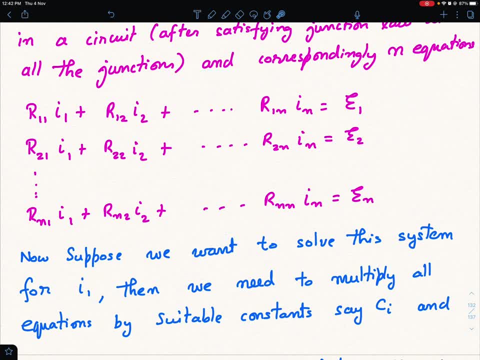 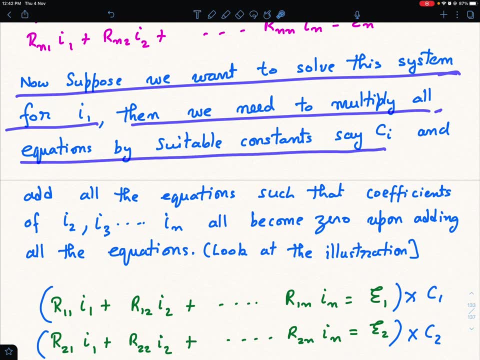 something. there will be some coefficient of I 1 and all other variables will be eliminated by if you multiply them with suitable constants. So that is what I have written. Suppose we want to solve the system of system for I 1, then we need to multiply all the equations by suitable constants. 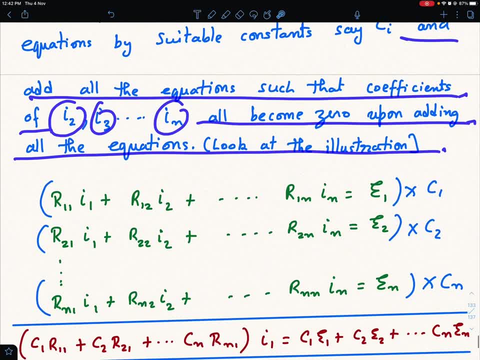 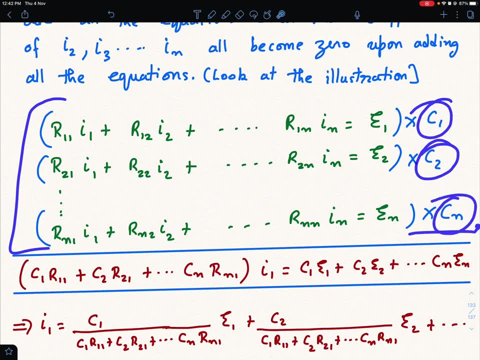 say C, i, and add all the equations such that coefficients of I, 2, I, 3, I, n all become 0 when adding all the equations. So I will multiply all the equations by suitable constants and then add all the equations. So let us look at this illustration. So the same system of equations, I. 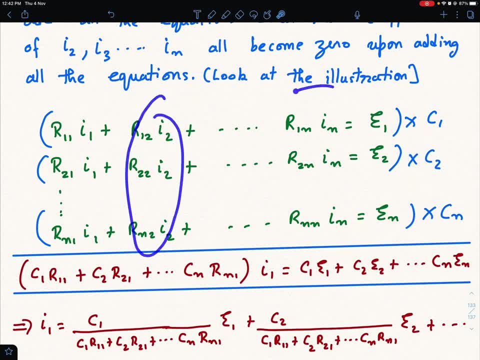 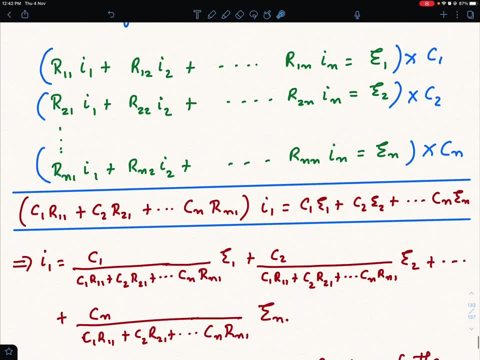 have copied. and let us say: these are the constants, and I am multiplying them, and these are chosen such that I 2 coefficient becomes 0 in the summation. I 3, I 4 and all of the way up to I n becomes 0, except for the coefficient of I 1.. So then, what will I get? So C 1 into R 1 1, C 2 into 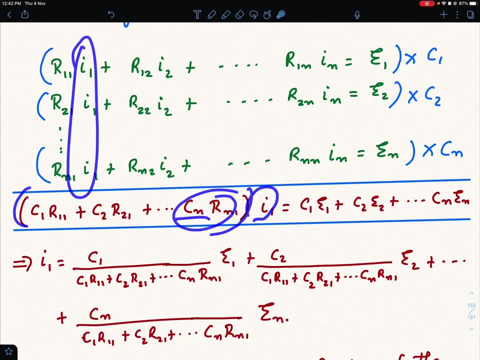 R 2, 1, and so on up to C n into R n 1. So C 1, 1, R 1 1, C 2, R n, 1, and so on up to C n into R n 1. So. 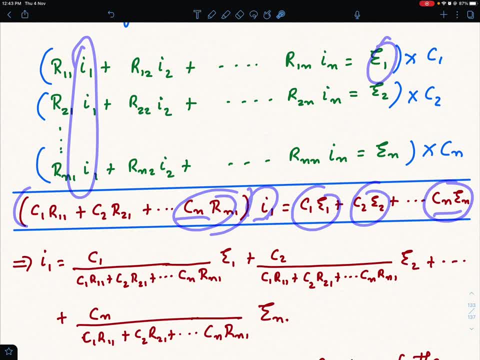 R 2, 1, C n, R, n, 1, whole thing multiplied by I 1 and this will be equal to, on the RHS, C 1, E 1, plus C 2, E, 2 and all the way up to C n, E, n. So what do I get for I 1? It will be C 1 divided by this. 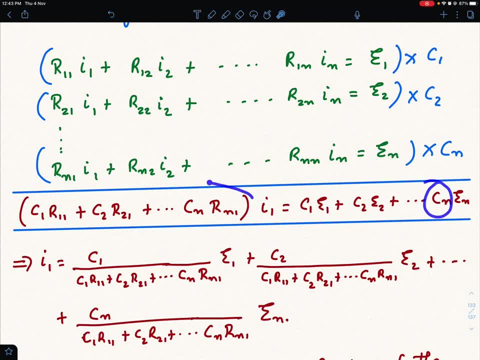 whole thing into E 1.. Similarly, plus C 2, divided by this whole thing into E 2, plus so on, up to C n divided by this whole thing into E n. So this is what we get. Okay, and now you can clear. 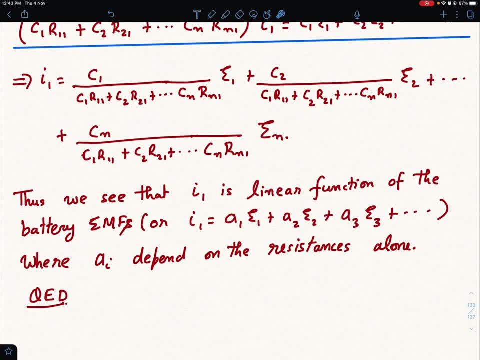 this, So you can clearly see that current I 1 is a linear combination of all the EMFs. Once again, there are no product terms like E 1, E 2 or square terms, even E 1 square, E 2, square 2. E 1- E 2. 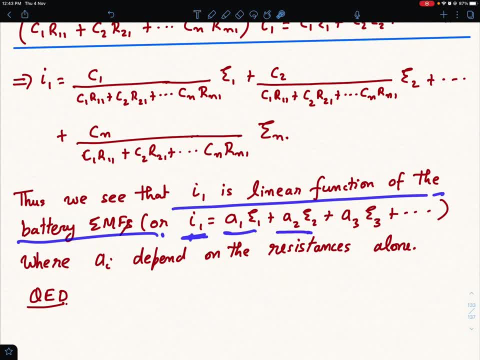 something like that is not there. Okay, So thus we see that I 1 is a linear function of battery EMFs. and what is this form? This is A 1 times E 1 plus A 2 times E 2 plus A 3 times E 3, where 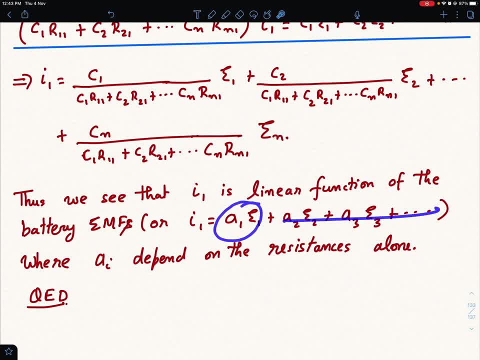 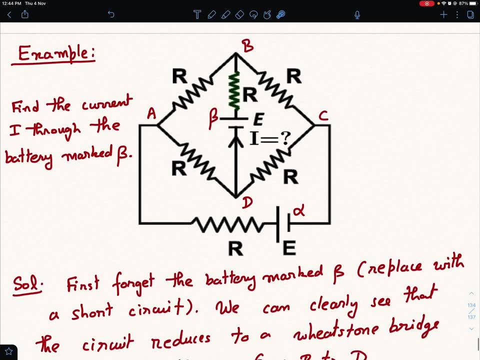 A. I depend on the resistances alone, and this is what I wanted to prove. So I can put: for getting this term, I can put all these terms to 0, and for getting the second term, I can put this and other terms to 0, and so on and add them up. Okay, So now I am going to present to you a. 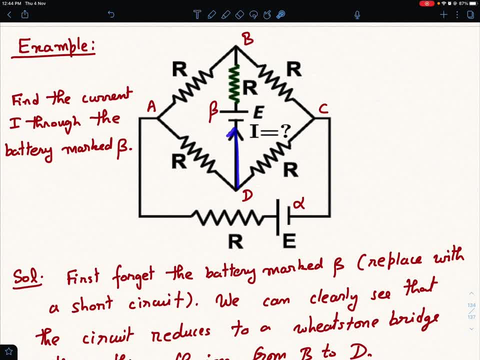 cute example. So here we have to find current I through the battery mark beta. So this is the battery mark beta and there is another battery mark alpha, and I want to find out the current through this battery. Okay, So what do I do? According to the superposition method, we can. 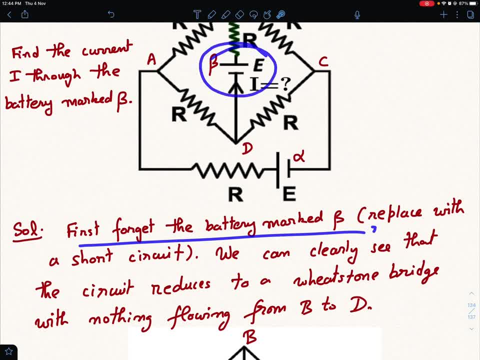 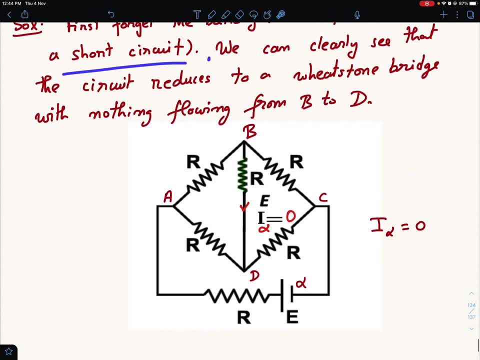 consider one battery at a time and replace the other battery by a short circuit. So let us first forget the battery mark beta. Let us forget this battery and replace it with a short circuit. Okay, You remove this battery and you connect it with a short circuit. So what does it look like? This is what your circuit looks. 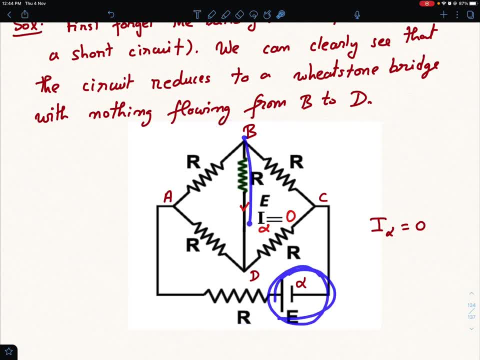 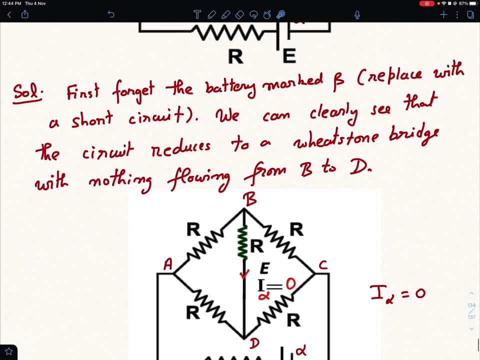 like when you remove this battery. and now something beautiful has happened. See, this is a Wheatstone bridge, Right. So because of this battery mark alpha, there is no current in the branch BD. Okay, So some simplification has happened. 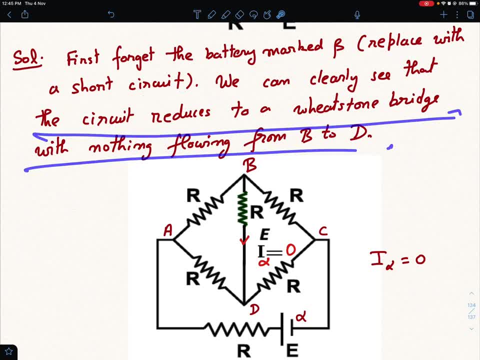 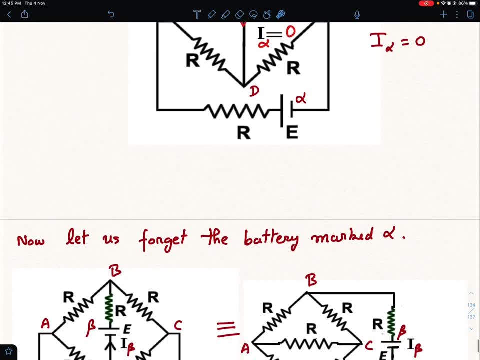 And the problem is now looking a little easier. Okay, So, first we forgot the battery mark beta and replaced it with a short circuit. We can clearly see that the circuit reduces to a Wheatstone bridge, with nothing flowing from B to D. Okay, So I, due to alpha is zero. 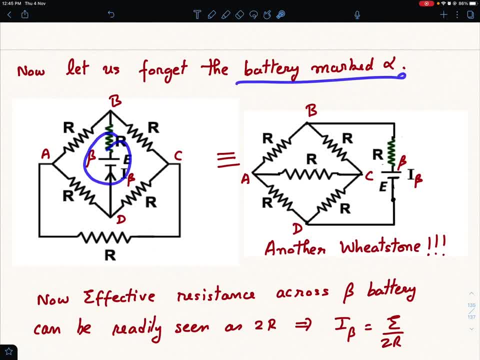 Okay, Now let us forget the battery mark alpha. Now I will forget the other battery, So I will forget this battery and then I will be having the only the battery mark beta. So this I have replaced by this battery I have removed by a short circuit. Okay, So, 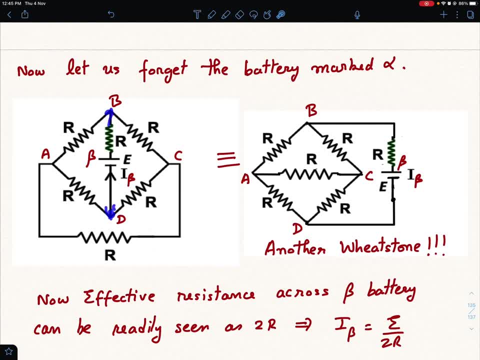 now I am having a battery mark beta. Now you see, in this there is a battery and resistor in series, connected between B and D, and this resistor is connected between A and C. So I have just rearranged this equation, rearranged this circuit to look like the circuit shown. 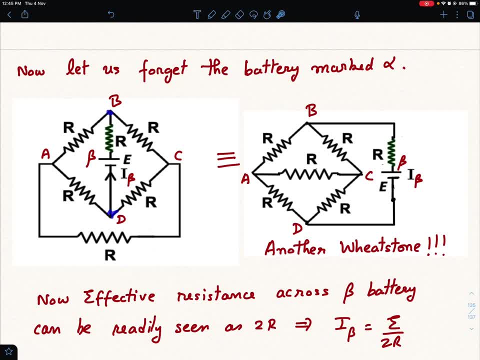 on the right hand side. Can you see that right hand side circuit is exactly same as the left hand side circuit, except I mean because between B and D you see this is the resistor, and so between resistor and battery combination. So here also you see resistor and battery. 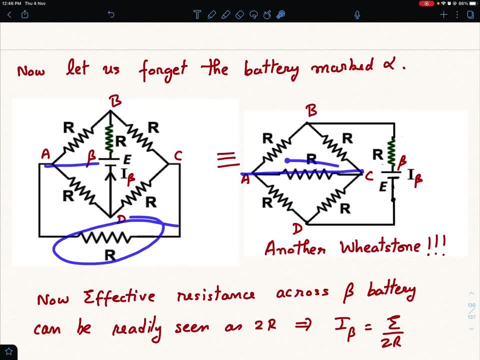 combination is there between B and D. So just, it is a same topology, just a little bit of rearrangement, and then this resistor is connected between A and C. So I have directly connected between A and C. So these two circuits are, from the topology point of view, exactly. 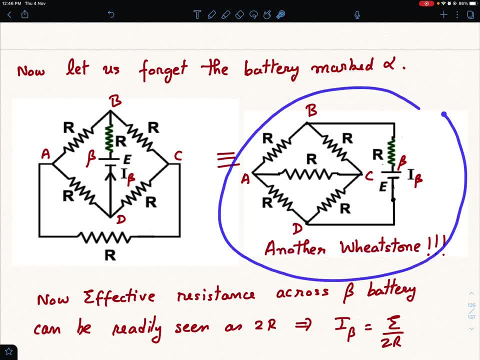 same circuits. Okay, And here again you can see this is another Wheatstone bridge. How beautiful is that There is another Wheatstone bridge. you can see, nothing is going to flow from A to C and now, and you know that the current is only due to this battery. now, Now. 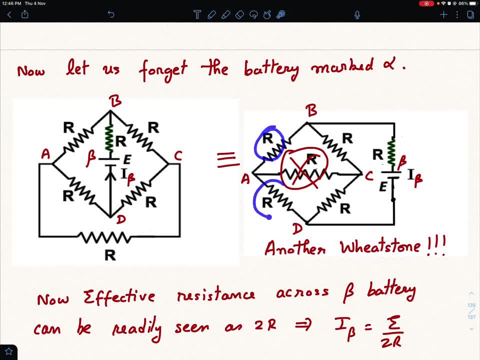 it is a simple circuit. you can as well forget this resistor. and then what is the effective resistance of this? if you see, So this is R and this is R, So two R in series and this is R, this is R, two R in series. and this two R, in parallel with this, two R becomes: 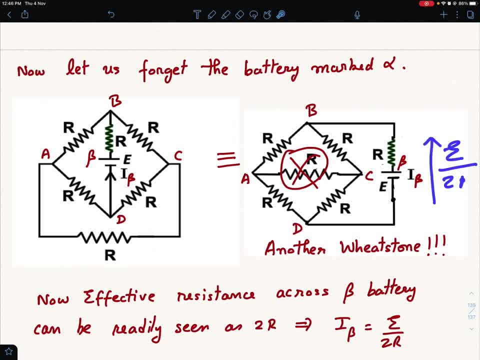 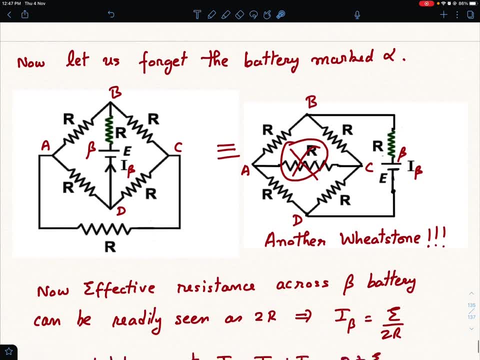 R, So this whole thing, whole resistance, becomes R, and this whole R is in series with this R. So therefore battery, So the current flowing through the battery will be simply E by two R, Okay, And and because of the other battery, there was no current through this branch. Okay, So that is what. 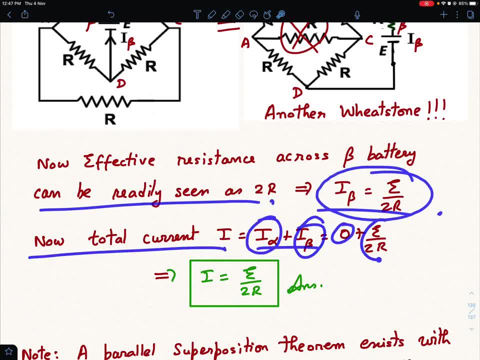 I have written. So effective resistance across beta battery can easily be seen as two R and I. beta is simply E by two R. So total current becomes I due to alpha plus I due to beta. that is, 0 plus E by two R. So that is our final answer. Okay, So this was the application. 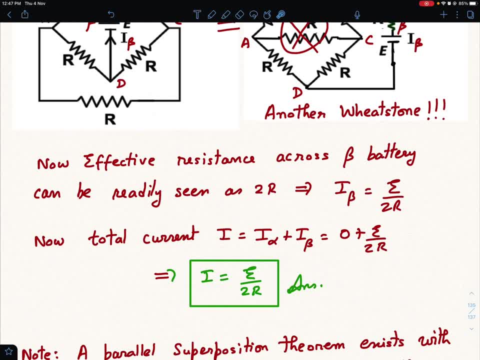 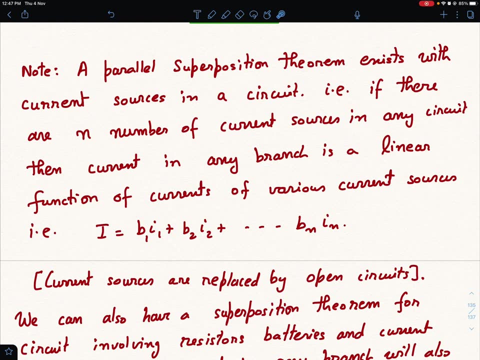 of superposition principle. Now there exist other superposition principles, also with current and mixture of current and battery, battery, current sources and batteries, but for JE purpose they are not very important. although I am going to state them, one or two problems might help you. 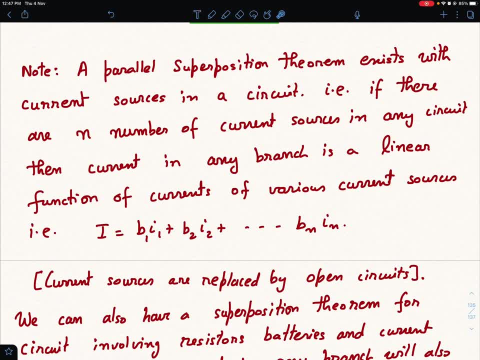 might get help by using those principles. like an Erudo, problem is there with infinite mesh of resistors. so there the method of proof will be on the same lines that I have done for the superposition, so I will just state the theorem. so a parallel superposition theorem exists with. 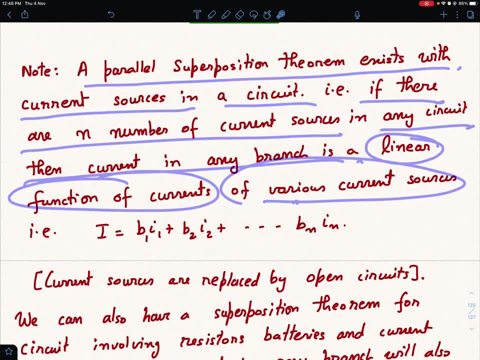 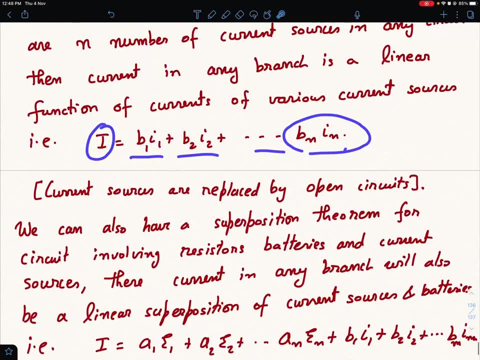 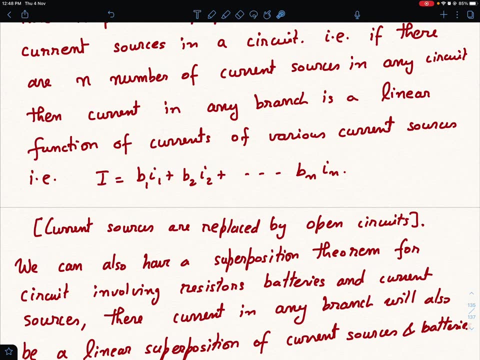 current sources in circuit. that is, if there are n number of current sources in any circuit, then current in any branch is linear function of the currents of various current sources. okay, so capital I is b1, i1 plus b2, i2 and so on, up to bn. in now, and please remember in mind, 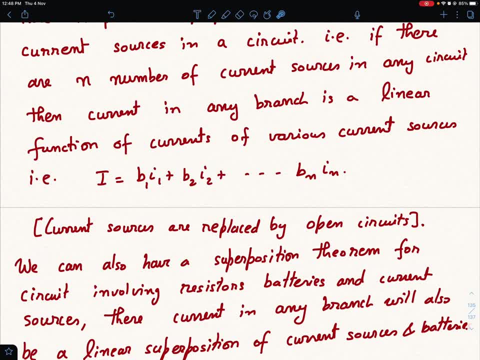 constant current sources. they should be replaced by open circuits. why? because what does it mean to have a constant current source? that means, let us say, I have a battery of one mole volts and then resistor of also of one mole ohms, so then that will supply a constant current of one ampere. right, because a small resistor like